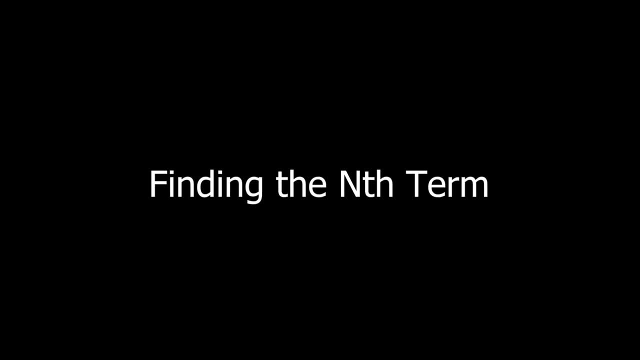 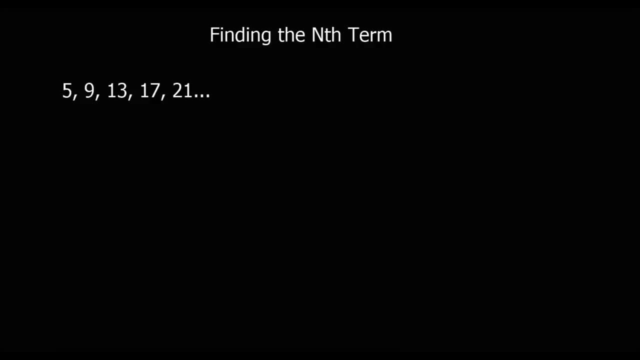 Here we're being asked to find the nth term, So we're going to find the rule for the sequence from the sequence. So the first thing we're going to look for is: what's the pattern here? what's going on? So it's 5, 9,, 13,, 17,, 21.. So it's going up in fours every time. 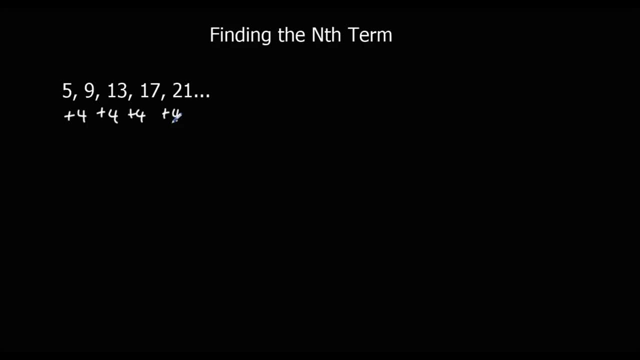 So the term to term rule is plus four every time. So if it's going up in fours we say it's 4n. So 4n is the four times table, It's four times one. So I'll write 4n up here. 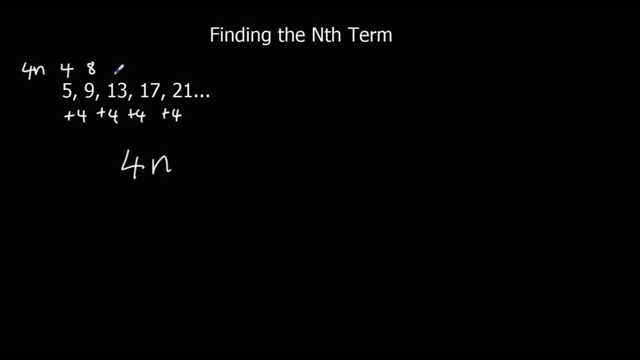 Four times one is four, Four times two is eight, And 12, 16, 20.. So that's the four times table. So it's related to the four times table. This is like the four times table, but it isn't the. 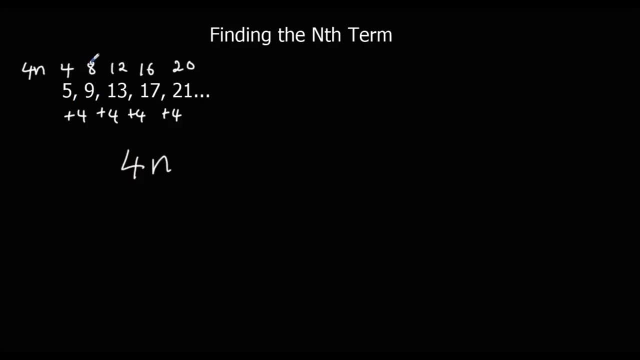 four times table. What's the difference between these? What have we got to do to the four times table to get this sequence? So it's always one bigger than the four times table. So if we add one onto the four times table, 4n plus one. that is our sequence. So the nth term is 4n plus one. 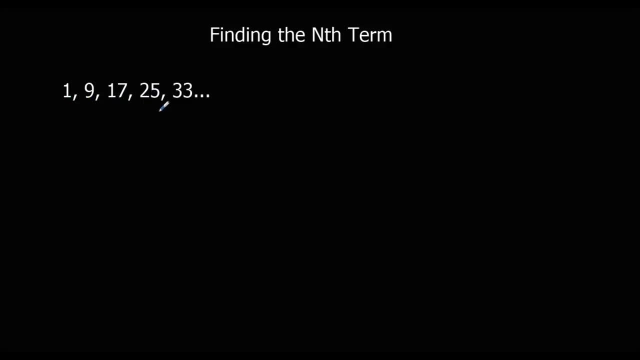 Okay, so here we've got 1,, 9,, 17,, 25, 33.. We're going to look at what's going on. What have we got to do every time? So it's plus eight every time. So what goes up in eighths is the eight. 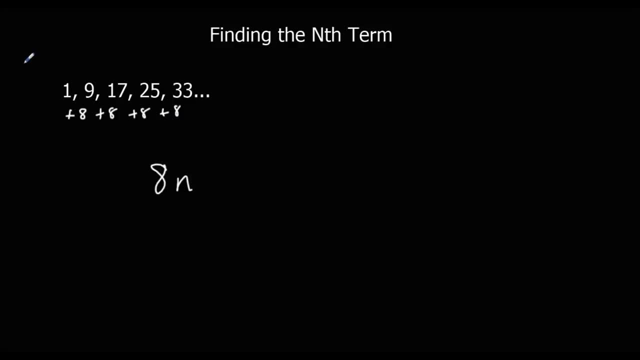 times table. It's 8n. So 8n is the eight times table. So 8,, 16,, 24,, 32, and 40.. The next question we've got to do to the eight times table to get to our sequence: What happens? So 8 to 1,. 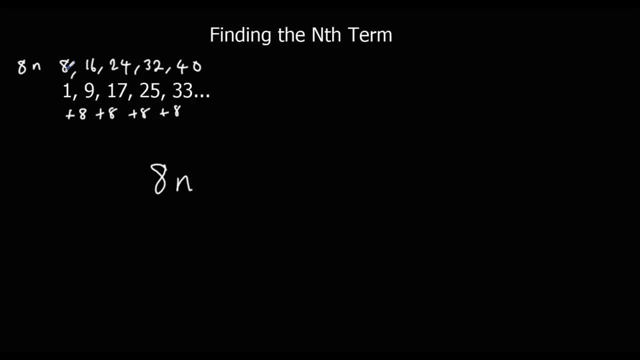 16 to 9.. What have we got to do? We've got to take away seven, So it's seven less. It's always seven less than the eight times table, So it's 8n minus seven. 8n. take away seven creates our. 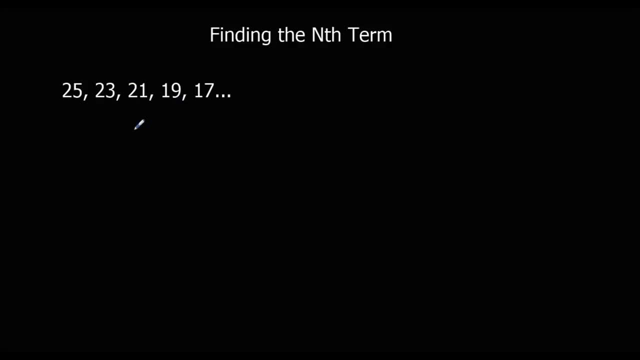 sequence: Okay, so this one's going down. So what have we got to do? every time It's take off two, So minus two every time. Minus two every time, So it's minus two, n this time The minus two times table, One times minus. 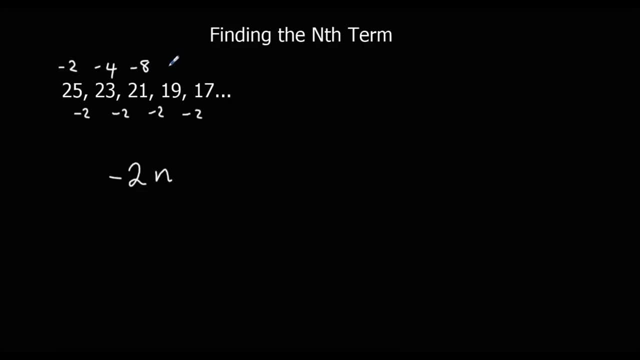 two, two times minus two, three, nope, Three times minus two, and so on. So what have we got to do to get from minus two n the minus two times table up to our sequence, It's always 27 higher. 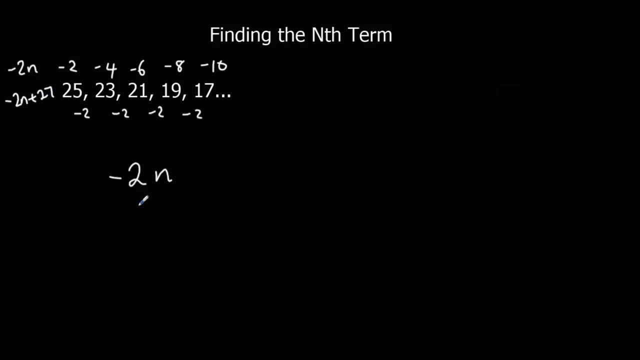 So minus two n, add on 27.. Or we could write it that way around: Minus two n, plus 27.. Or we could write 27 minus two n. Either one of those either one of those are right. Okay, here's some sequences. 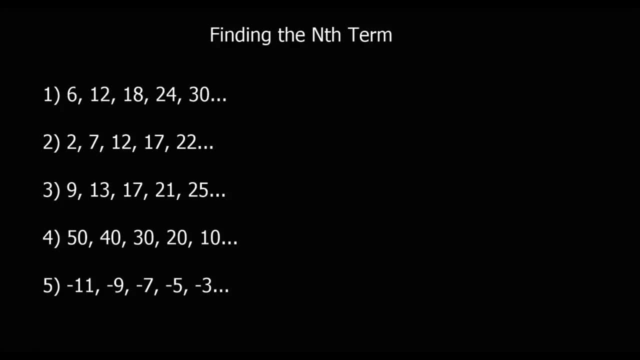 for you to try, So pause the video, give them a go and I'll put the answers up afterwards. Okay, so the first one is going up in sixes, So it's six n. It actually is the six times table, So we don't have to do anything. to six n. The answer is: 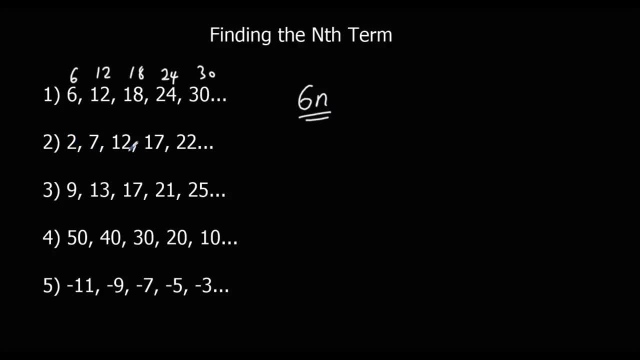 just six n by itself. Second one: we're going up in fives, So it's the five times table. five n Five, 10, 15,, 20, 25.. What have we got to do to the five times table to get our sequence? 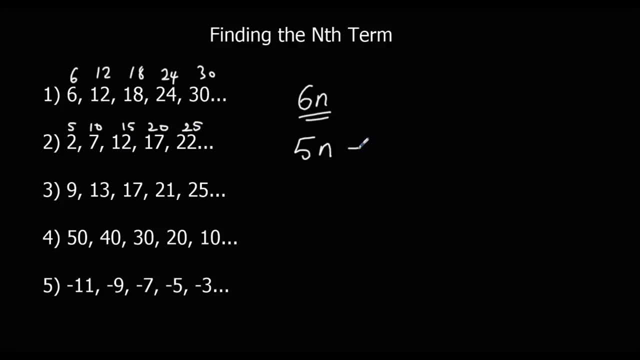 Take off three. Three less every time, Three less every time. So take off three. The next one: we're going up in fours every time, So it's gonna be four n. That's four, eight, 12,, 16,, 20.. What have we got to do to the four times table to get this? 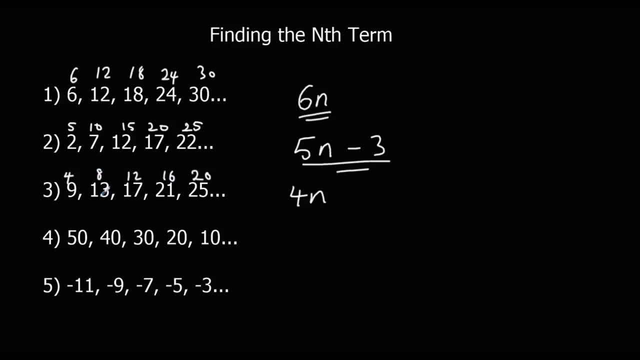 to get this sequence, Add on five, Five more every time, So it's the four times table plus five. Four n plus five. This one's going down in tens Minus 10 every time, So it's minus 10 n. 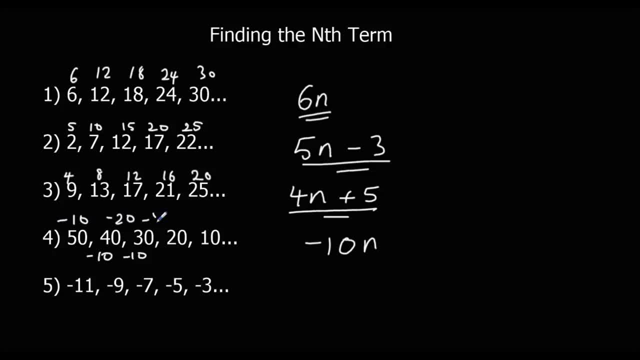 So minus 10 n. So it's minus 10 n Minus 10 n. So it's minus 10 n. So it's minus 10 n Minus 10 n minus 10. timetable Minus 30, minus 40,, minus 50.. What we've got to do to get from minus.